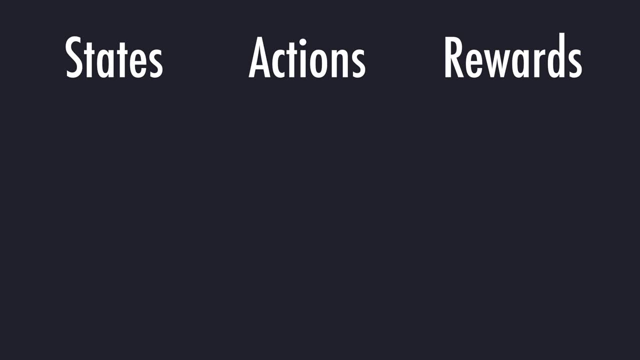 transitioning into a new state. the reward you receive and perhaps even the action selection are not deterministic but have a certain probability. Imagine the following: Your agent is a plumber with a mustache, He is in this position here and he wants to go one step upwards In the first initial. 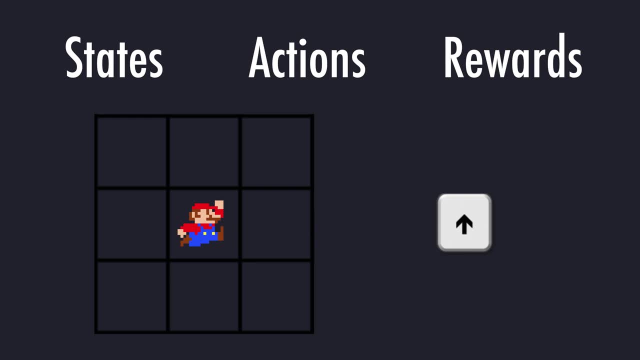 state, for example, s0, he wants to take the action. a0 is equal to north or up, But he then slips and doesn't move into field 2, but moves into field 4.. Now, don't get scared. the following will: 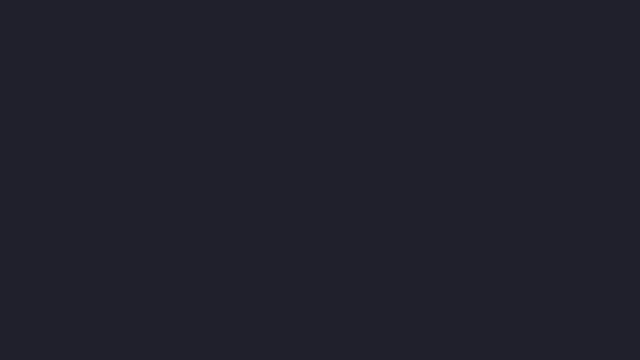 look worse than it is. I'll repeat myself a few times so it hopefully makes more sense. Here you can see the formal definition of a Markov decision process. You might have seen this in your lecture. The graph and this mathematical representation are really the same thing, but the important. 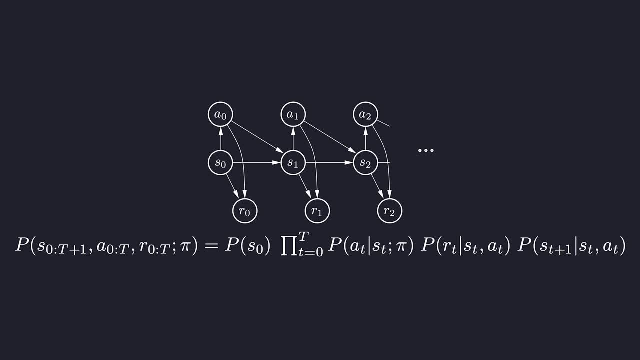 thing to understand is the graph. This graph is not a state transfer graph like in automatons. This is an illustration which shows random variables and how they depend on each other. We, for example, have this variable s0 for the world's initial state. 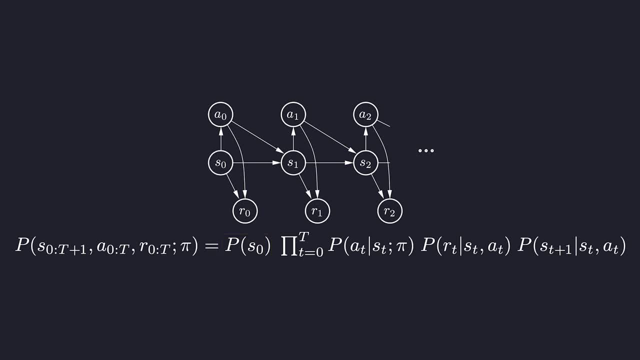 Which is also probabilistic and unknown. This does actually make sense. Just imagine a robot that is placed somewhere in a room. How would the robot know where it was dropped? Then there is the state, st plus one, which also has a certain probability of being the actual envisioned. 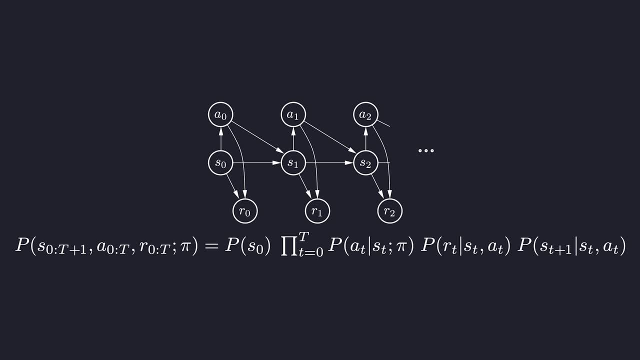 next state. Remember the plumber example. Receiving a reward is also probabilistic and the selection of the action can theoretically also be, But this one actually isn't most case deterministic. So your policy pi will definitely predict one next action to take based on the current state. This whole scary formula here is just the formal way of writing. 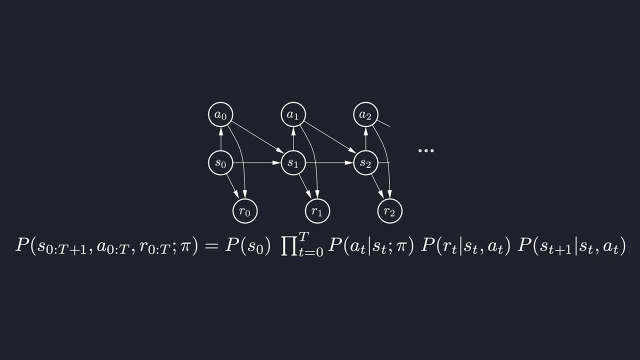 down all individual probabilities combined. Now for the graph. This probability, for example, which is the probability, or rather the probability distribution, of getting into state s1 when, is represented by these two arrows. It shows state s1 is conditionally dependent on the variables s0 and a0.. And s1 is not conditionally dependent of actions that happen in the future. 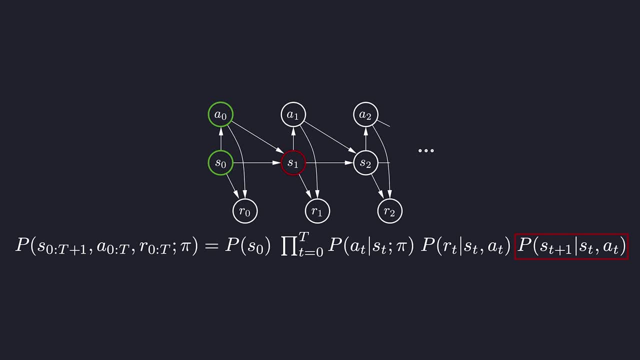 This is also how our real world works. The next action is not dependent on future ones, Otherwise our current concept of time would be not really true and all over the place. But yeah, let's continue with that. So the time step t is not only used to illustrate the order of actions or states, etc. but can 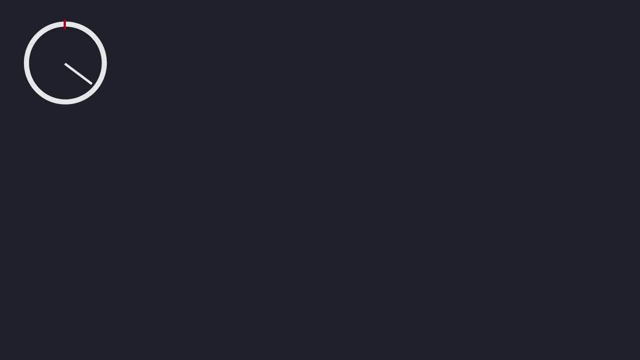 also be viewed as an absolute dependency of time. For example, a rocket has to land on a planet at a specific time. Those are then called non-stationary MDPs, But in most cases the absolute time is not really important, So we often just have a stationary MDP with. 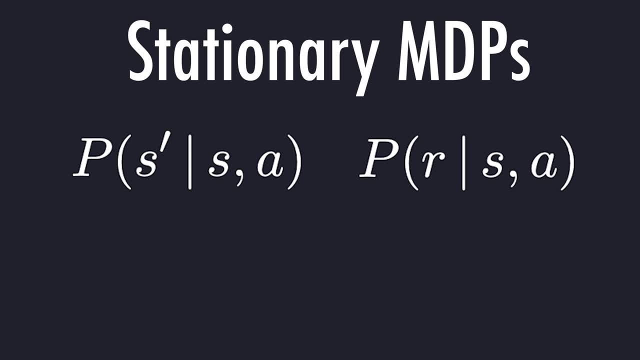 always one transition and return, So let's take a look at the probability distribution for each state. To go even further, We often don't even really care about the actual probability distribution of the rewards we could get in state s when choosing action a, But we just always use 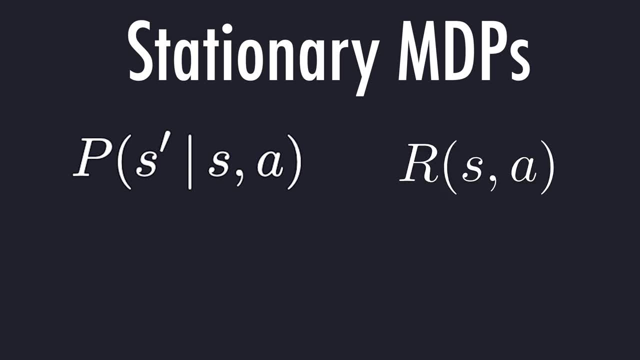 the average reward, Which is then notated like this, with the big R. So to recap, We have states which describe the world in a specific moment. Then we have actions that are deterministic and can be selected from a domain. So we have states which describe the world in a specific moment. Then we have actions that are deterministic and can be selected from a domain. 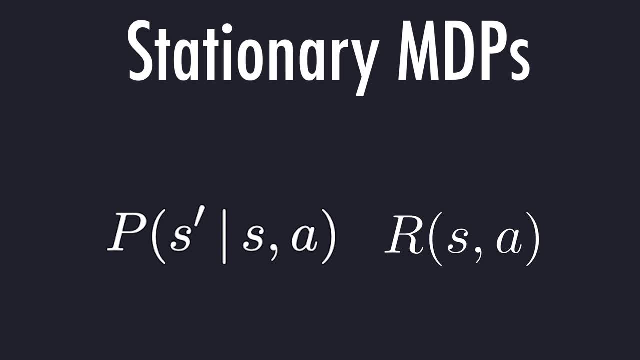 So we have states which describe the world in a specific moment. Then we have actions that are deterministic and can be selected from a domain. The probabilities of entering state st plus one when choosing action 80 in state st are independent of time, For example, always when you are in the same state s and want to go left. 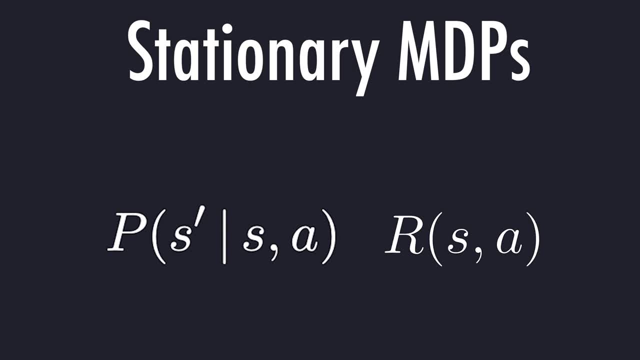 you could have a 90% chance of actually doing so and 10% chance of slipping and going right. Finally, we have rewards that are dependent on the state and the action chosen. We can have multiple different rewards with certain probabilities, but we really only care. 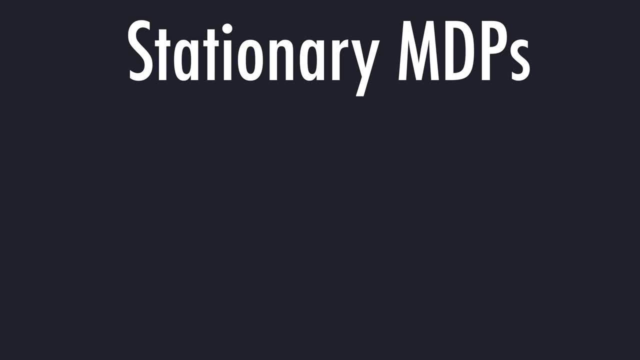 about the average reward. Now, all this is nice and cool, but this is just the definition of a problem setting. What would this mean practically? As you can probably imagine, with such general definitions, there are multiple ways of defining it for a specific case and there are different goals. 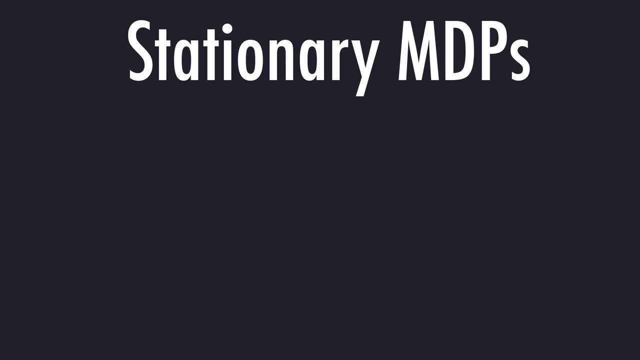 you want to achieve in your specific case. But if we look at such a stationary and discrete Markov decision process on a simple level, all the necessary probabilities are just simple t's. This means you would have a table for p of s zero, or it could simply be one deterministic. 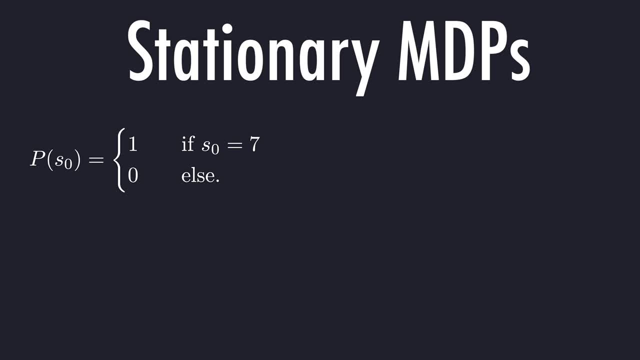 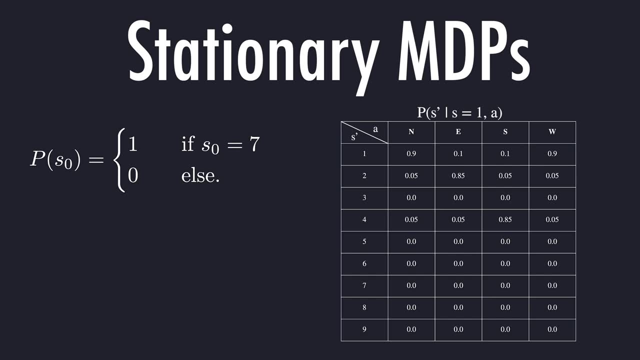 starting state, You would have a table for the transition probability when starting in s equal one, for example, which could look something like this: You would then have multiple such tables for each state s, and they will tell you the probabilities of getting to s prime when choosing. 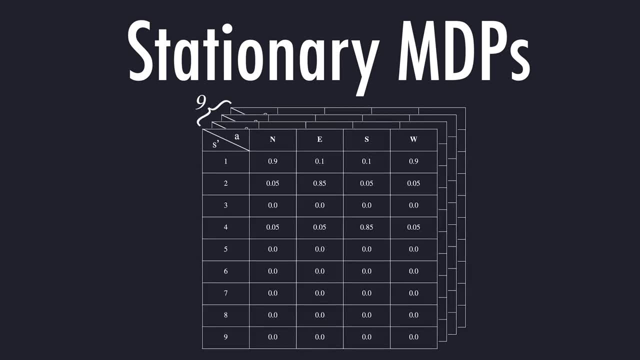 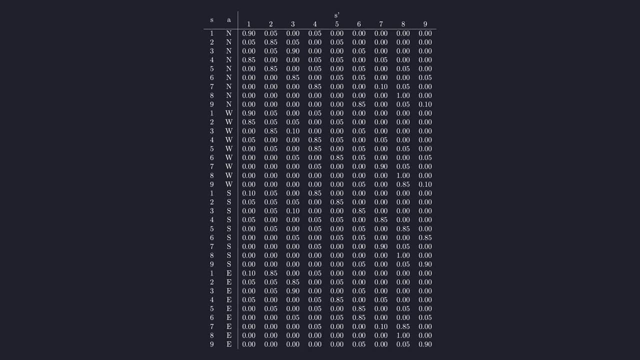 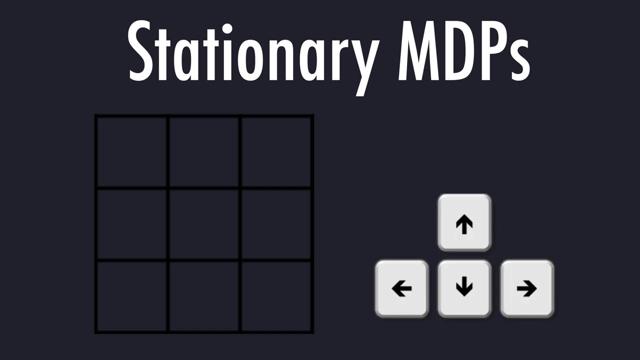 action a, But you don't need multiple tables like such. You can also select a table for each state. You can also store them in a tensor or all-in-one thought through table layout, but I think that would be very messy. For example, imagine again this setting here and you can go north, east. 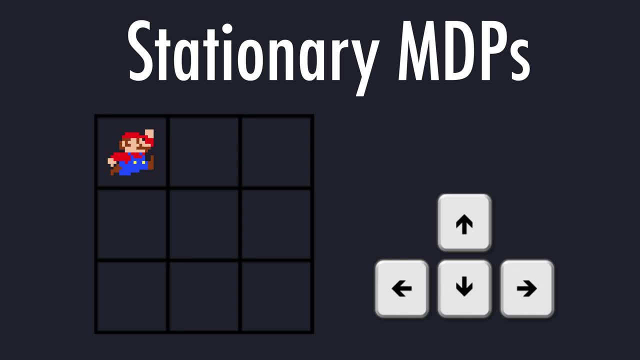 south west. If you now start at position one, you can go, for example, east and land on field two, but will succeed with only 85 percent, and the other 15 percent will split up to the other options. In this case, the only other option is that you land on field four. 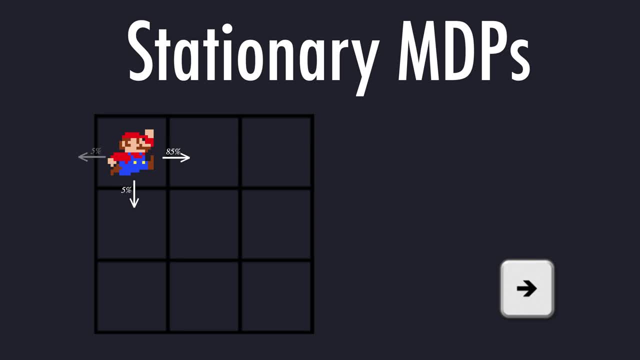 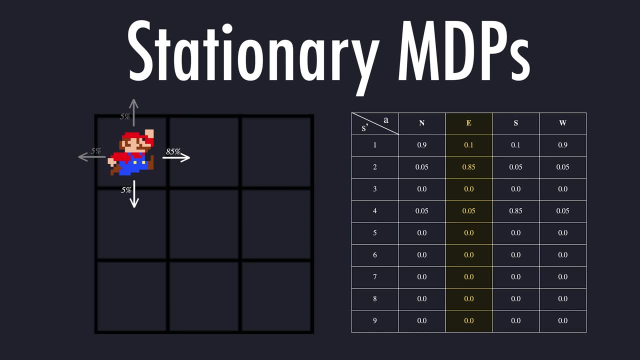 So that would be five percent. or to crash into the west wall and the north wall, which would let you not move at all and come out to be 10 percent of actually staying in the same place. We'll get to that example more in depth in a bit. You'll then also have a table with the average rewards. 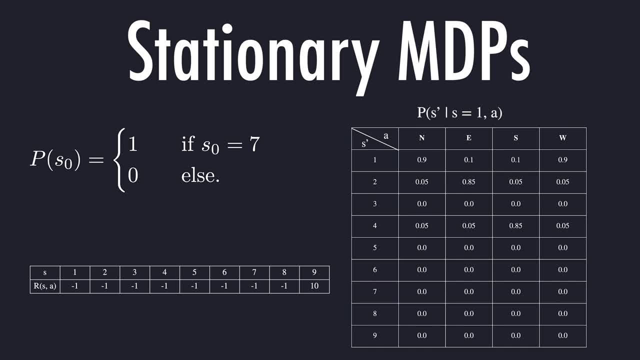 Again, those are tables that can be stored in any format. The goal of your algorithm is then to find the perfect policy, So to optimally decide which action a to take in the state s. Of course, optimally always depends on your definition, and then also on parameters. but 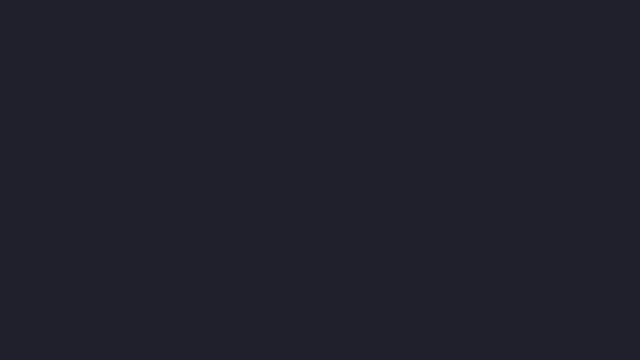 everything at its time. We'll finish this video with a little example exercise, which will require us to write down explicitly the probability and reward tables we just looked at For this three times three maze. that defines the respective mark of decision process, And here you can also. 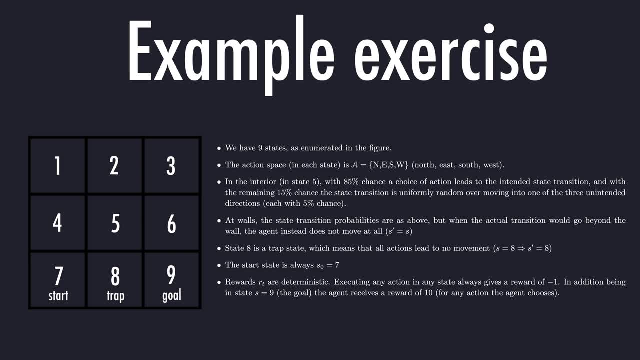 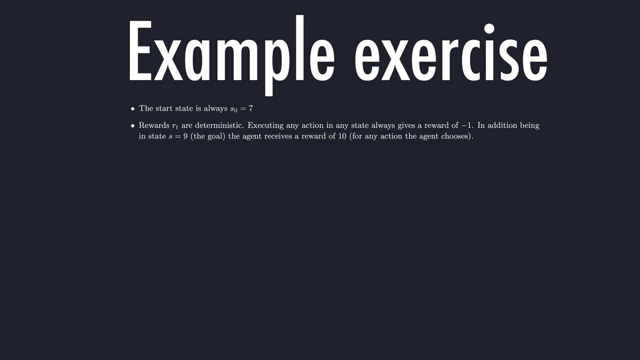 see the rules for the MDP. You can pause the video whenever you want and try to think about transition for a few states yourself. It shouldn't be too hard to get the hang of it. So let's start with the distribution of the initial state and rewards. Since they are deterministic, we can say the 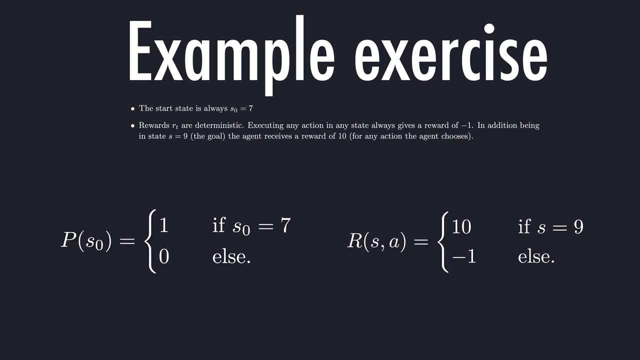 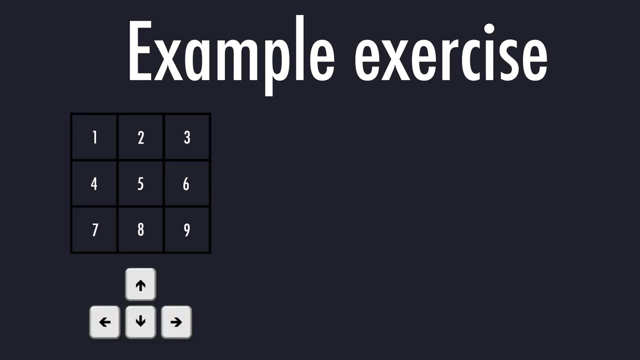 following for the initial state and reward. The mathematical expression can be simply put into a table with one column or row For the state transitions. let's look at one starting state together and I'll then show you the probabilities for every other state so you can compare it if you.